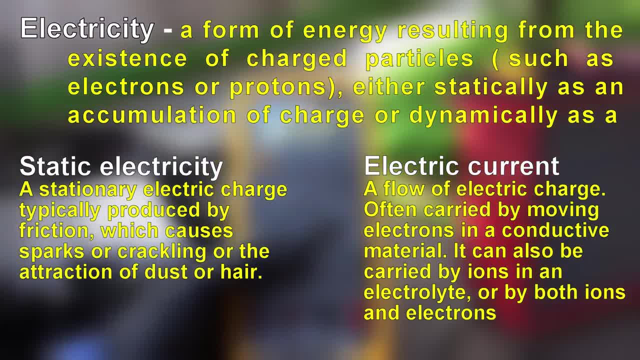 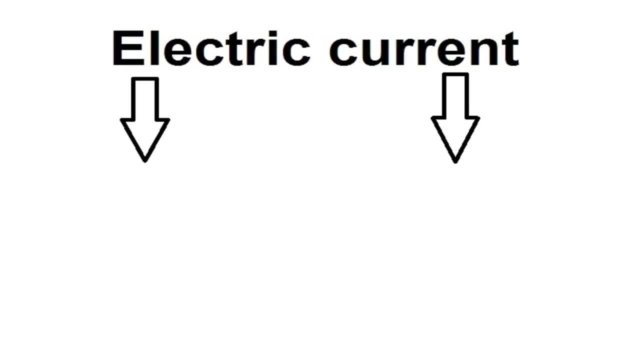 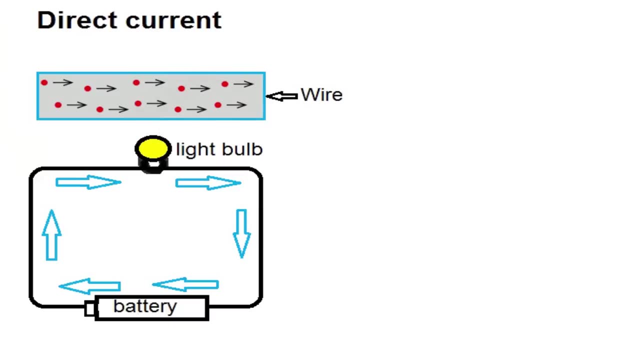 electricity. If the electrons are moving on a conductive material, then we call it electric current. When it comes to multimeters, we only talk about electric current. There are two types of electric current: DC current and AC current. DC means direct current, means the direction of the current always flows in one direction. 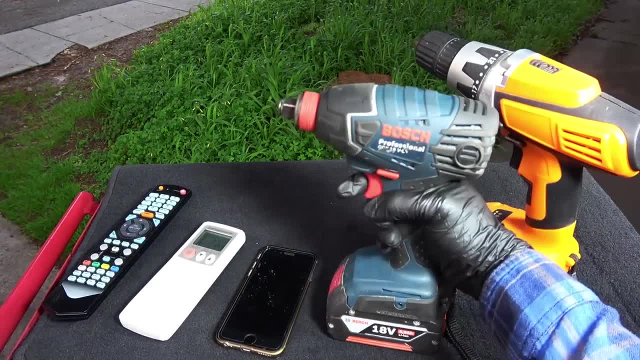 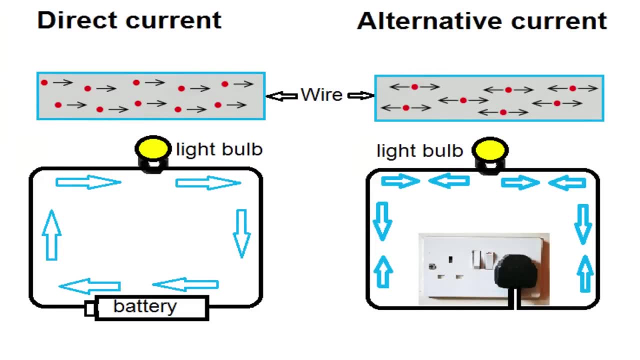 For example, any device that runs off of a battery is run by DC current. Next up we have the AC current. AC means alternative current, where the direction of the current always change. For example, the current coming through your wall outlet is AC current, so is most of the appliances you connect to it. 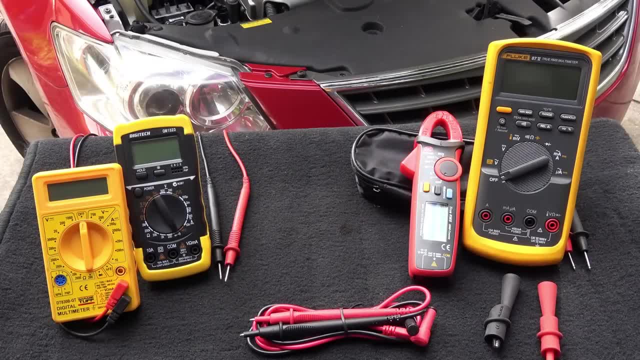 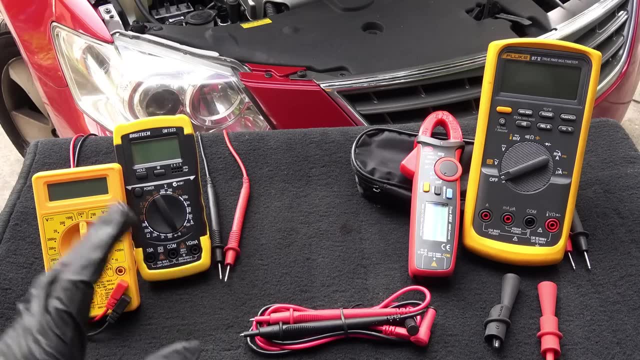 Now let's have a look at multimeters. There are two types of multimeters: manual range multimeters and auto range multimeters. Whatever multimeter you buy, they always come with at least two leads. One is red and one is black. 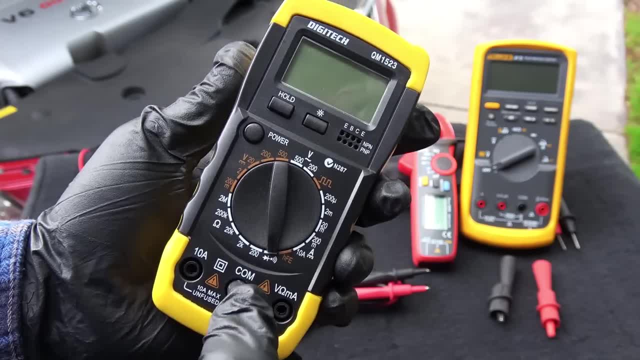 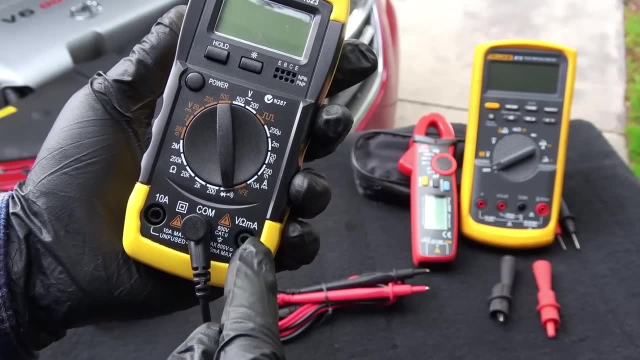 The black lead always goes to the common jack where it says common. The red lead goes to either of these two jacks, depending on what you are measuring. If you are measuring volts, resistance or milliamps, then you unplug the red light. 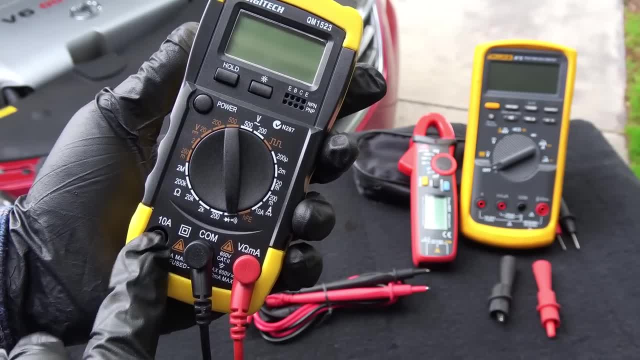 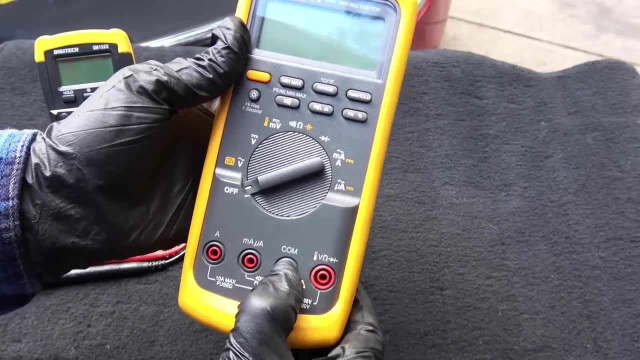 The red lead goes to this jack. If you are measuring larger currents, up to 10 amps, then the red lead goes here. Different multimeters may have different setup for the red jack. For example, in this multimeter. if you are testing volts, resistance or diodes, then the red lead goes here. 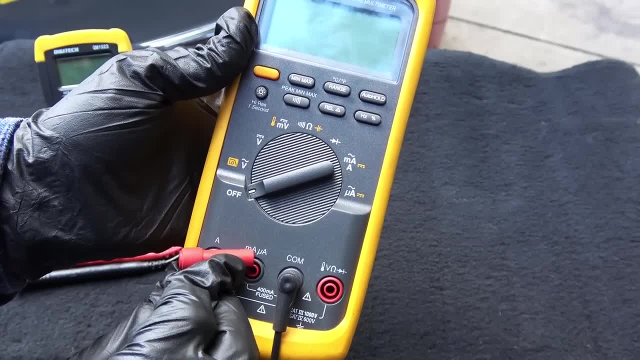 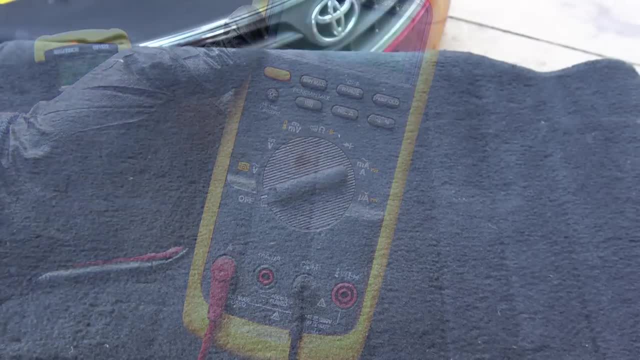 If you are testing smaller currents in milliamps or microamps, then the red lead goes here. For larger currents up to 10 amps, then the red lead goes here. First we will take a look at a very cheap manual range multimeter. 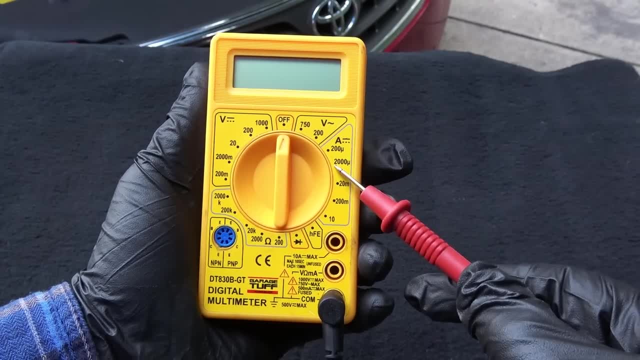 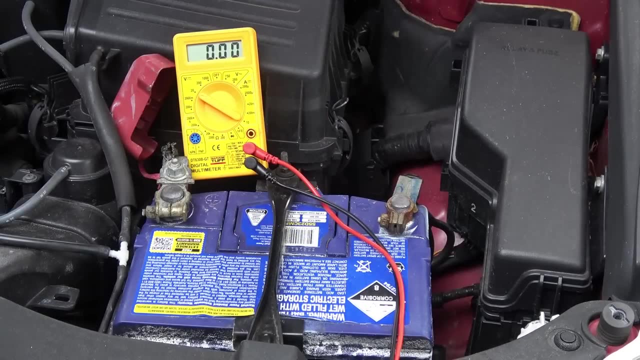 We are going to be looking at DC1.. We have AC voltage, AMPS, resistance and continuity. Let's start with DC voltage. I'm going to test this car barrier to see if it's good. So you need to have the red lead in this jack where it says volt. 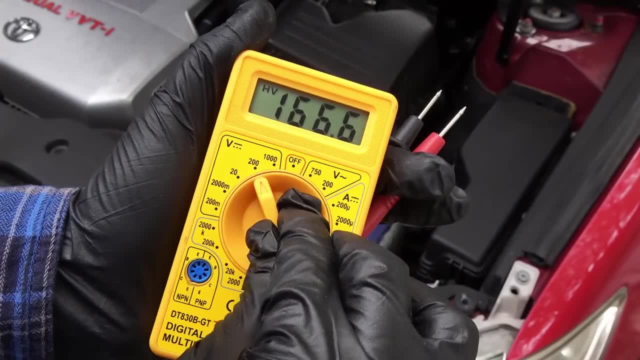 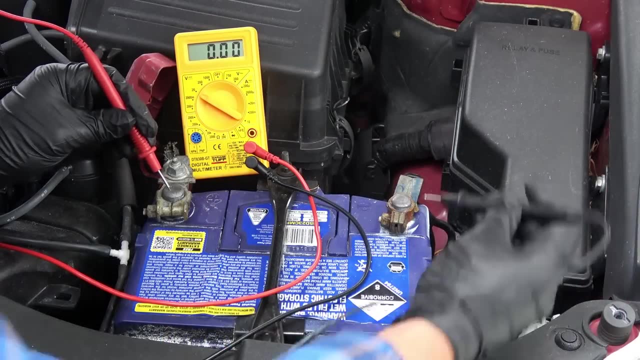 Because the car barriers are in 12 volts range, you want to turn the dial into the next number up from 12.. So in this multimeter, 20 is the closest number up from 12.. Then you want to connect the red lead to the positive terminal. 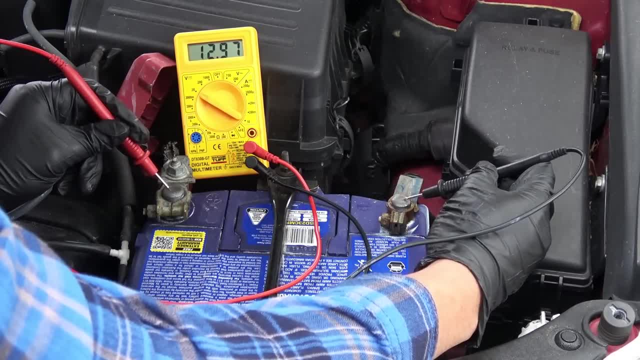 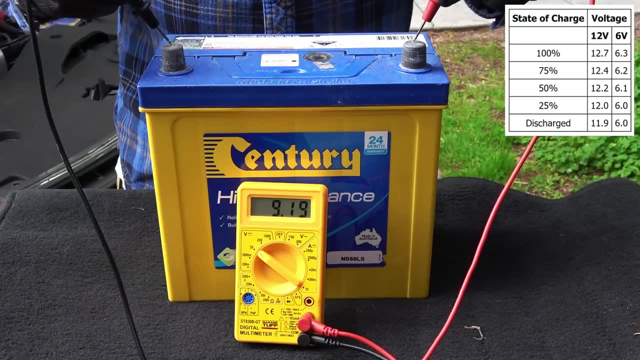 And the black lead to the negative terminal. We have 12.91 volts volts here and that is a good rating. If the rating was very low, then you definitely have a weak battery and you wanna replace it. Let's say you connect the leads backwards, it's not gonna do any damage. but the rating on the 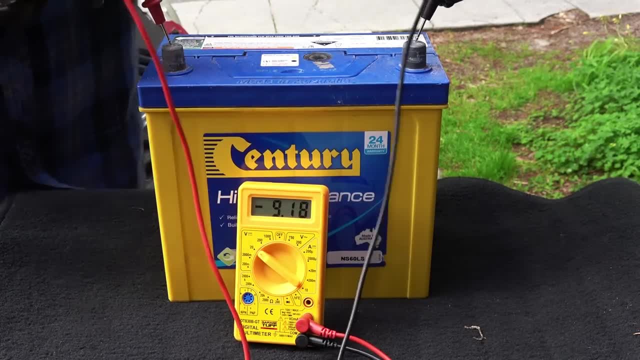 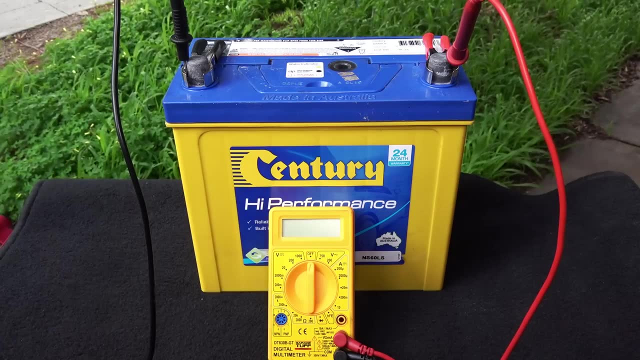 multimeter will be negative, letting you know that the current is flowing the other direction. that way you can identify the polarity, which is handy. Let's say you don't know the amount of voltage you wanna measure. well then, you always wanna start from the highest number available in your multimeter and 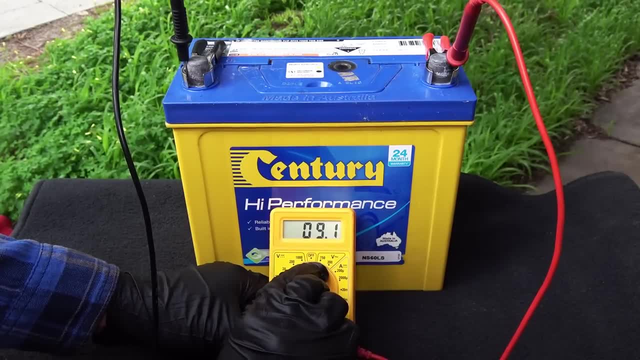 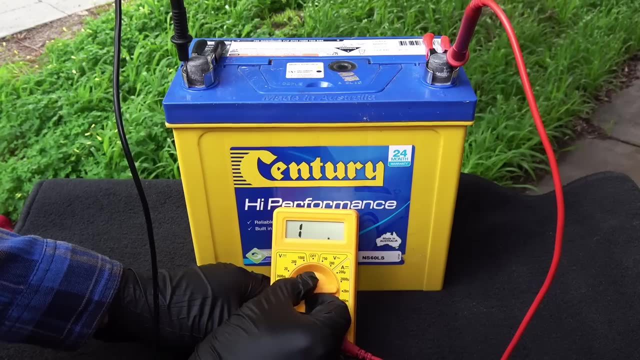 work your way down until you get an accurate rating. When I say an accurate rating, a rating with two decimals is accurate enough for most cases. If you get a rating of 1, that means the voltage you're gonna measure is beyond the selected range of your multimeter. so you wanna scale up until you get two decimal. 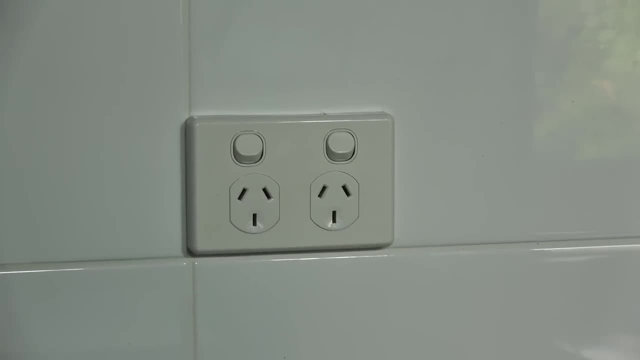 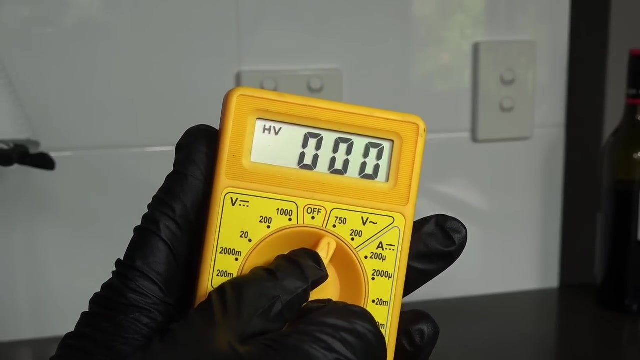 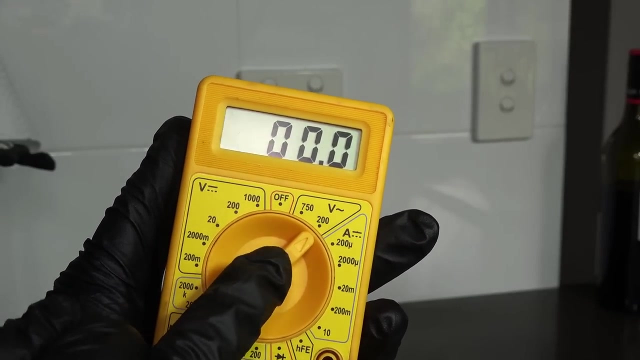 places. Let's move on to AC voltage. Let's see if this wall outlet is working. Now you wanna turn the dial into AC volts and we have two ratings: one is 200 volts and one is 750 volts. now, if you turn the dial into 200 volts, then the multimeter will only read up to 200.. that is good. 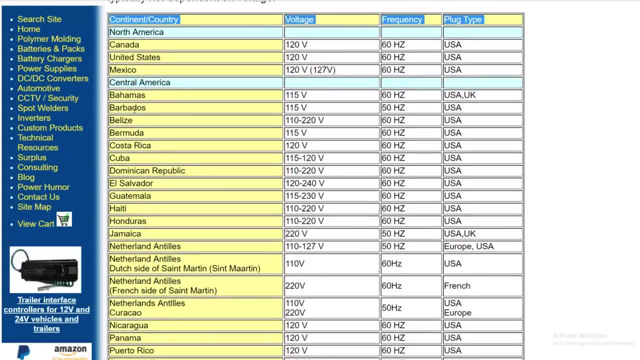 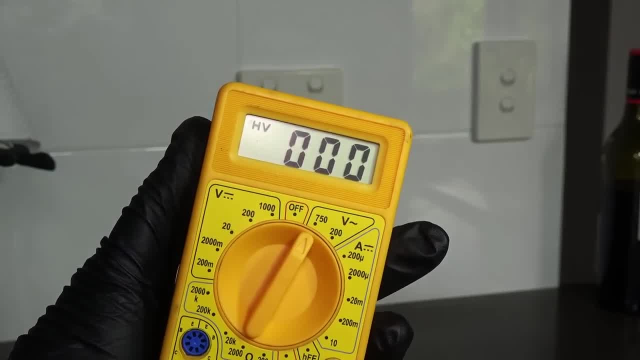 if you live in a country where household voltage is in 115 range, but in australia wall outlets have 240 volts, so i'm going to turn the dial into 750, because that is the next one up we have on this multimeter. you want to be careful when you're doing this: you don't touch these metal tips of. 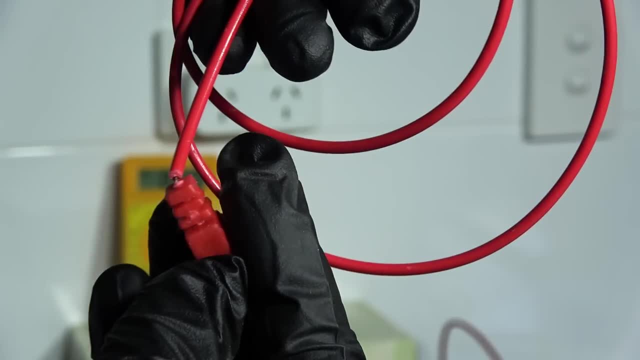 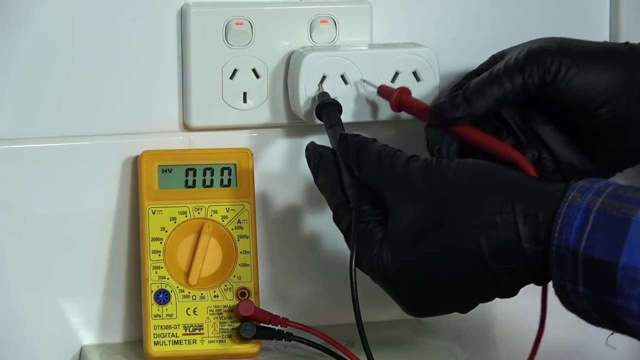 the probes. and also you want to make sure your test leads are not damaged or having any exposed wires, because you're dealing with high voltage and you don't want to get electrocuted. then you want to probe into the outlet and we have 240 volts. let's move on to measuring resistance. 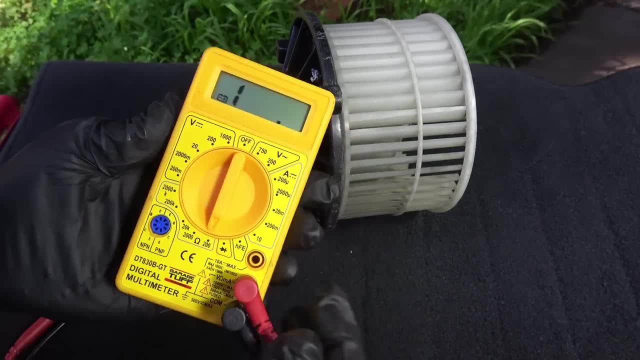 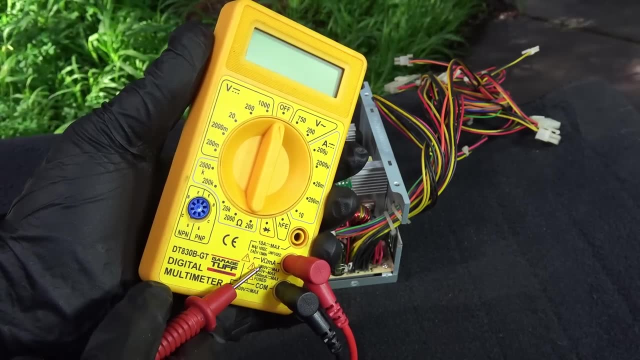 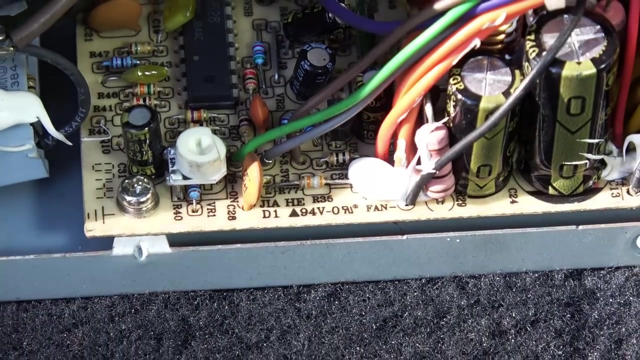 this is very easy. all you have to do is to turn the dial into resistance. this horseshoe mark right here is the standard symbol for the resistance, and if you look down here, the red list stays in the same place, because this jack can read resistance as well. resistance means how hard it is for the current to flow through in a circuit. 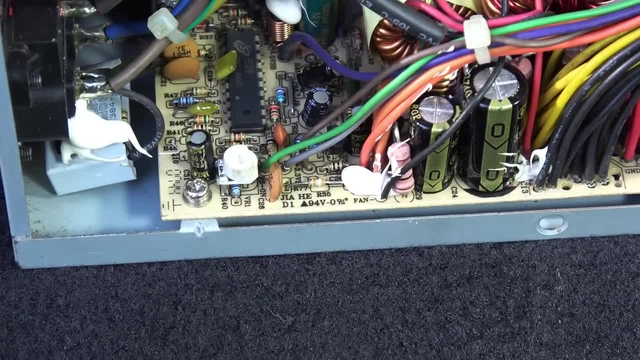 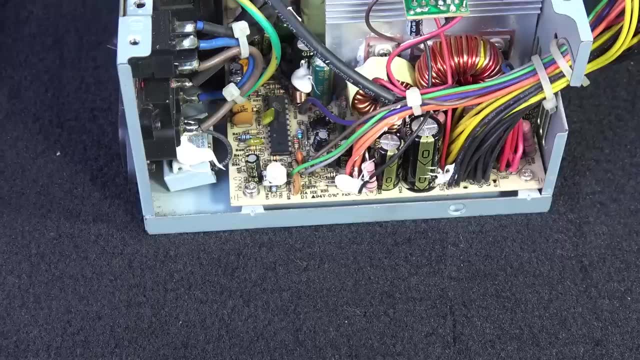 so let's say you measure the resistance of something while it is still connected to a power source or still connected to a circuit board, then the multimeter will take a different path, with the least resistance between the test leads and will give you a false reading. so whenever you test resistance, 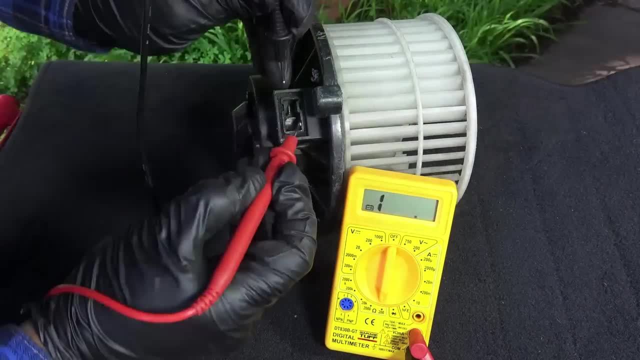 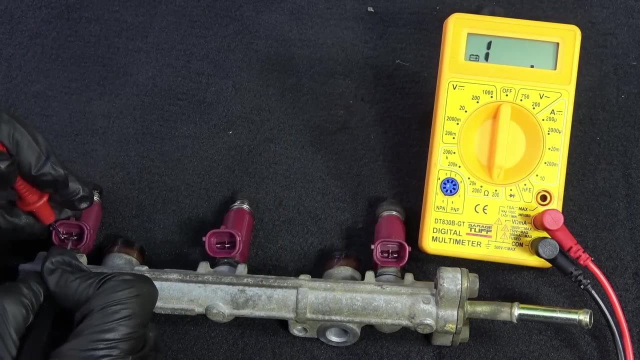 you always want to isolate the subject you're trying to work on. here i'm measuring the resistance of a blower motor. here i'm measuring the resistance of a fuel injector. now here's a practical example. let's say one of the fuel injectors in your car went out- a brand new one. 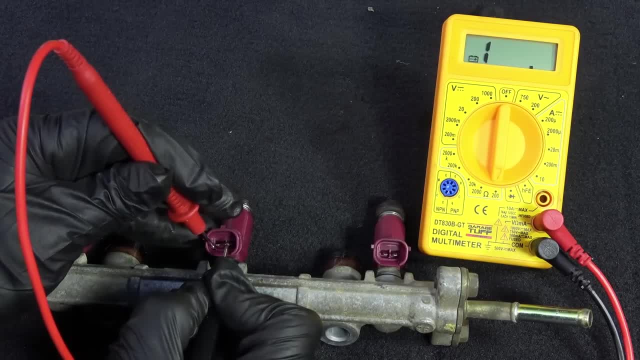 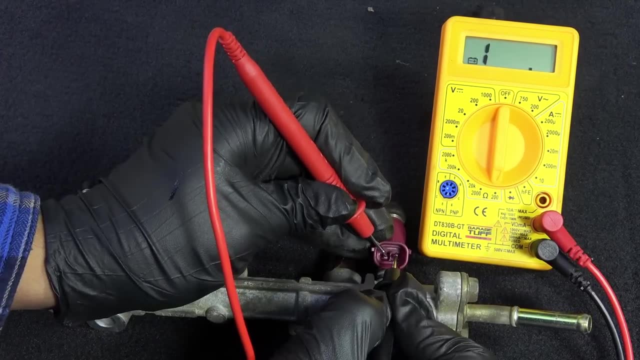 it's often very expensive. so let's say you're thinking about buying a used one from a junkyard, then the only way you can figure out whether this is a good one or a bad one is to check the resistance and see if the rating meets the manufacturer's specs. if the rating is different, 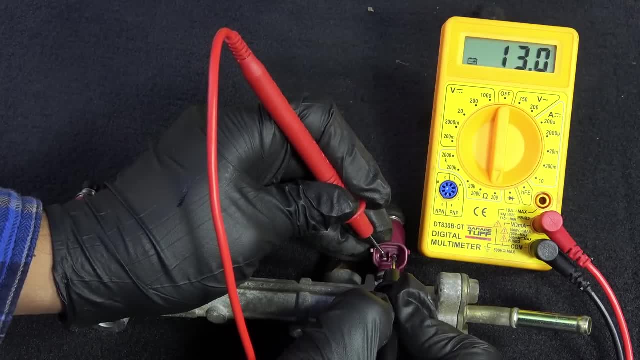 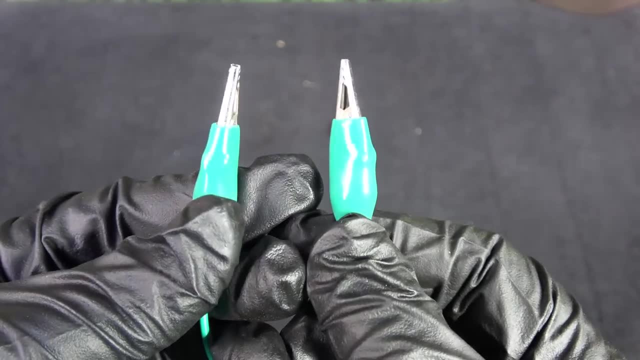 than what is mentioned in the specs. that means you're looking at a bad injector, so you look for another one. next up, we have the continuity. you can use this function to see if you have continuity between two points. if you have continuity, then the multimeter will beep. 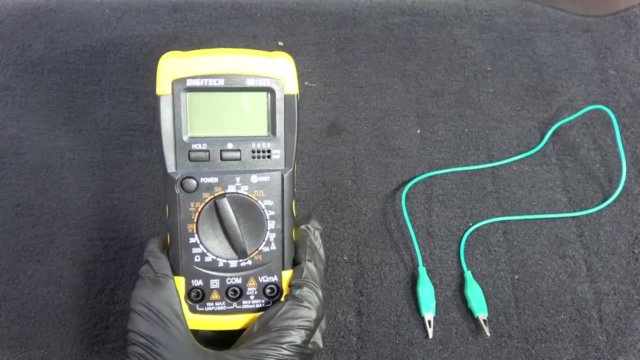 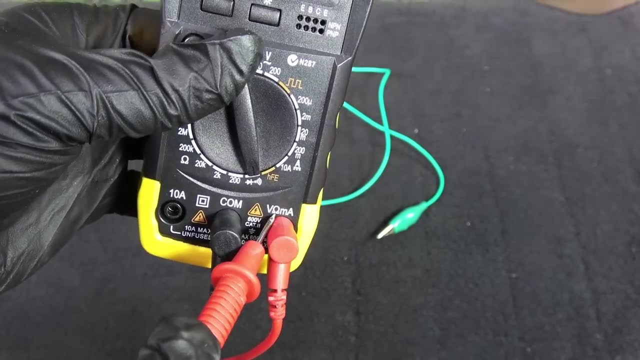 this cheap multimeter does not have a beep function, so let's move on to this one. now you can turn the dial into this symbol that looks like a speaker. that is continuity, and the red list still stays in the same place where it says resistance. let's see if this piece of wire 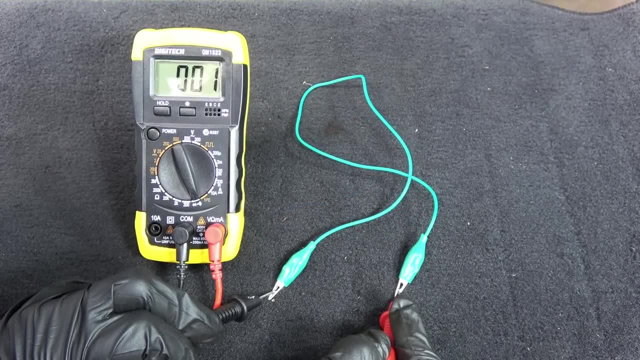 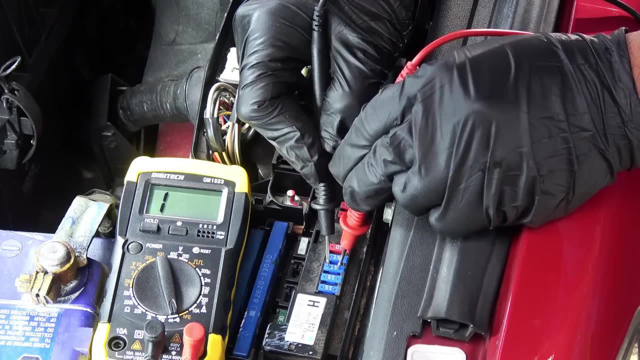 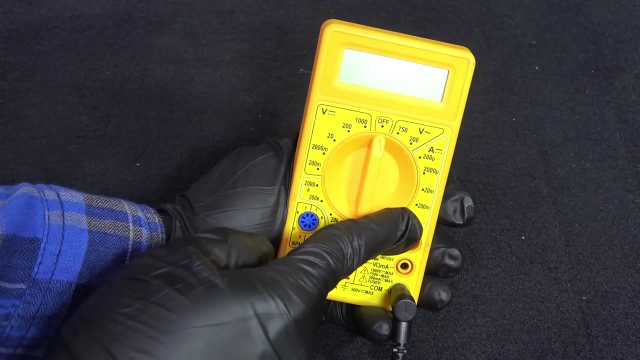 is broken. we hear the beep, so this wire is good. here i'm testing the fuses in my car to see if i have burn fuse. here i'm testing an earphone. finally, let's move on to measuring current. if you are measuring milliamps, then the red. 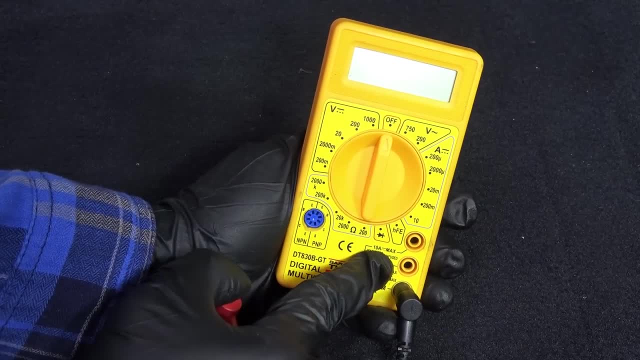 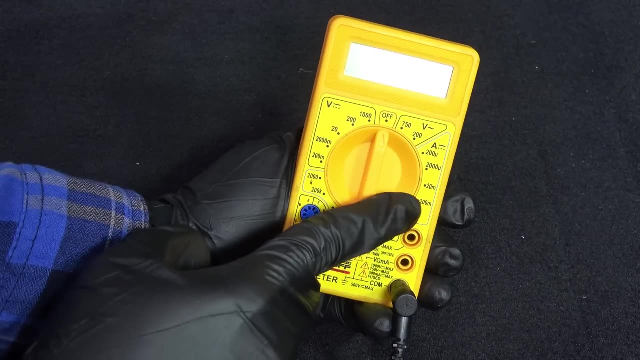 lead stays in here. if you are measuring larger currents, up to 10 names, then the red lead goes here. if you are not sure about how much current you're going to measure, then always start from the amps instead of milliamps. that way you wouldn't damage your multimeter and if the 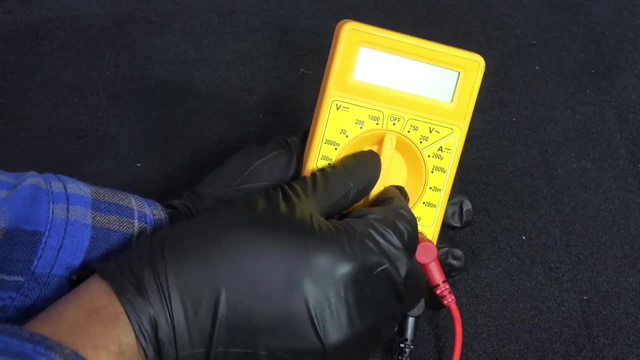 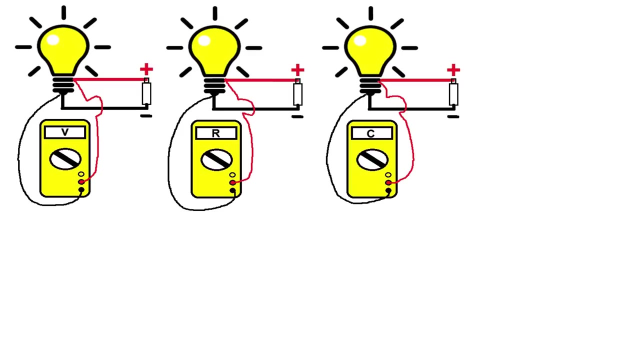 reading is actually in very low amps. then you can move on to milliamps for more accuracy. now, unlike measuring volts, resistance or continuity, where we place the test leads in parallel to the flow, now we are displacing: the test leads in series with the flow. here's an example. 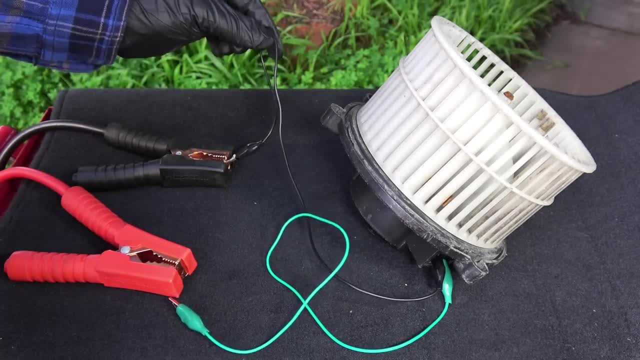 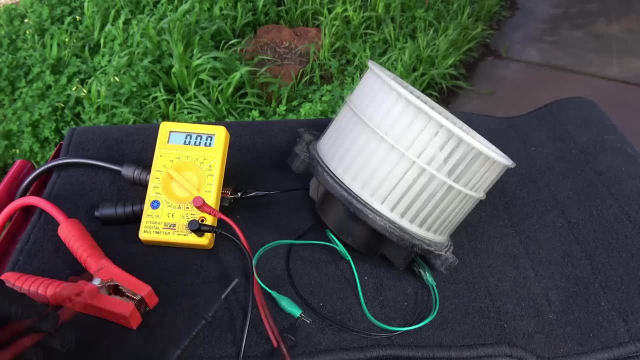 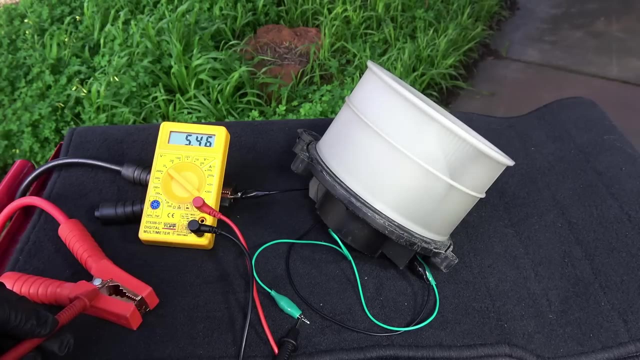 of a fan connected to a battery. here we have the negative side and here we have the positive side. to measure amps, here we have the multimeters placed into the power side wire and, as you can see, we have a reading of 5.5 amps. now let me show you something real quick. as you can see, when the motor first started to spin, it draws a lot of current. now it is normal to draw a little more current in the beginning, but too much current means the motor is very hard to spin, which is a little bit tricky, and this could be the reason why your car's fuse for the blower motor keeps. 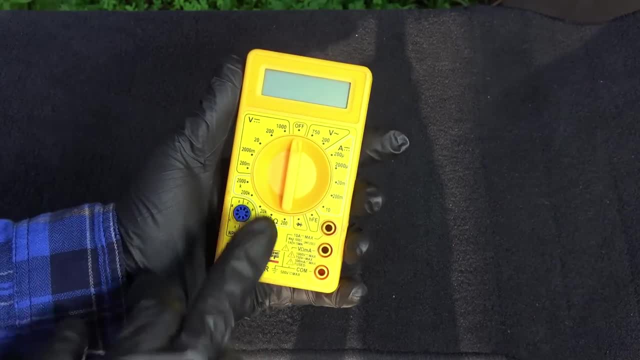 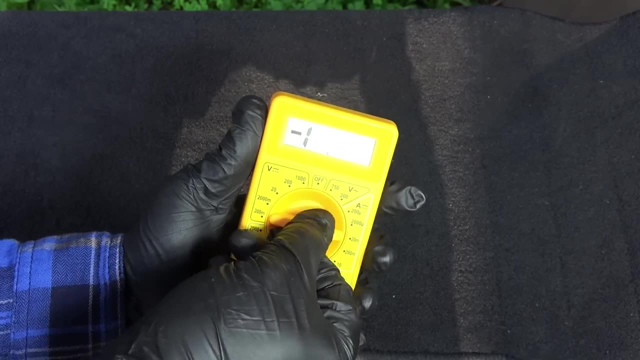 blowing once in a while. all right now. that's how you properly use a multimeter for basic functions. the only downside is that when you're using a manual range multimeter like this, you always have to turn the dial into different settings. so if you're thinking about buying a multimeter, 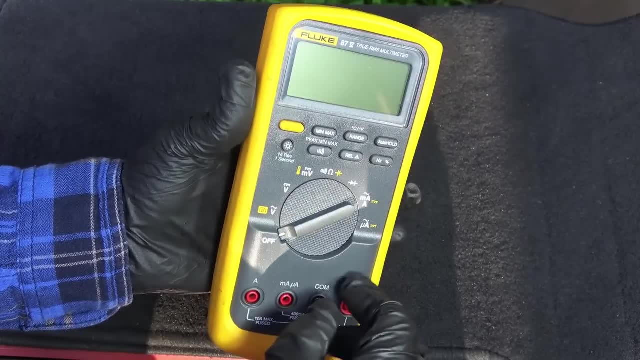 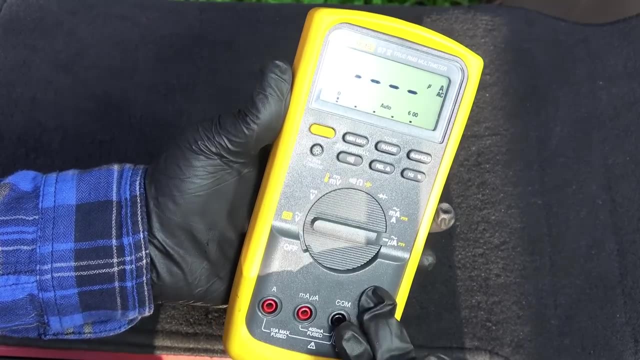 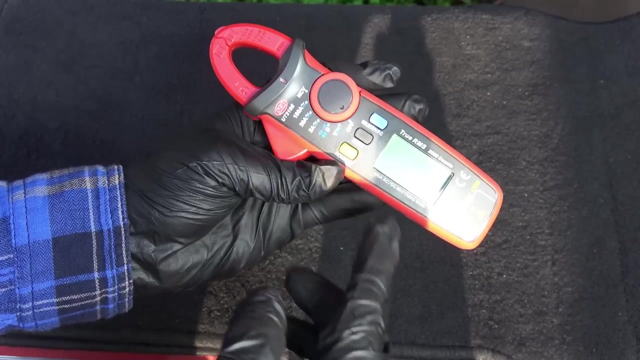 make sure you buy an auto range multimeter. you just have to select what you're going to measure- ac voltage, dc voltage, resistance, continuity, amps- and start measuring me. this is going to make your life that much easier, and if you're going to be using your multimeter all the time to measure amps, then you can think about buying a multimeter with an amp. 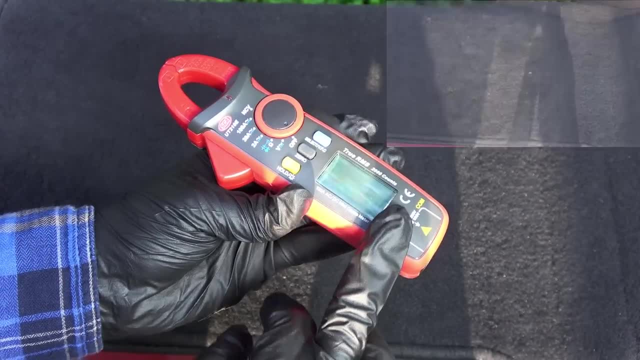 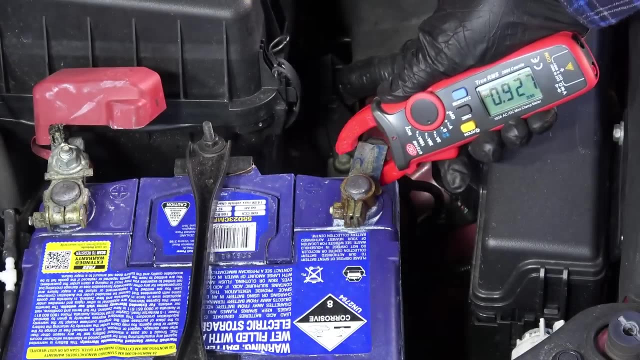 clamp. this has all the basic functions of a multimeter. it has two jacks for the test leads, but when you're measuring amps, rather than splicing in your multimeter and messing around with the wires, you can easily clamp it over the wire and get the reading for regular users there. 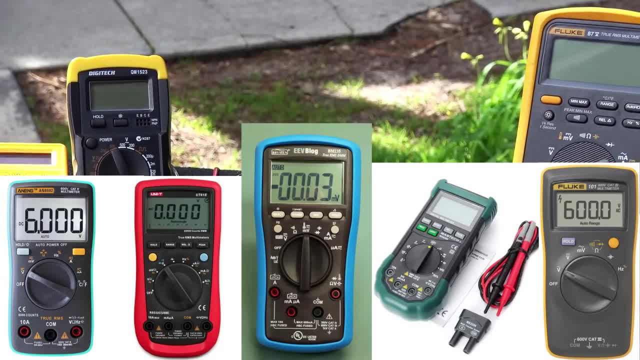 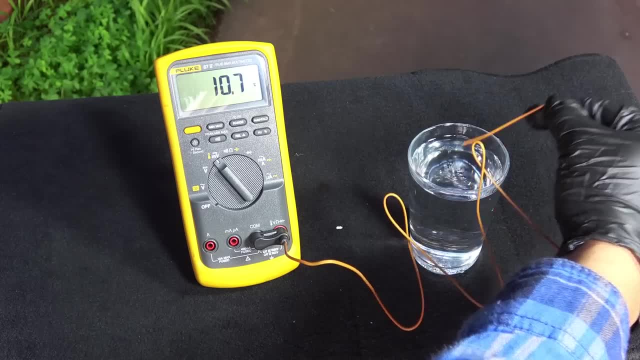 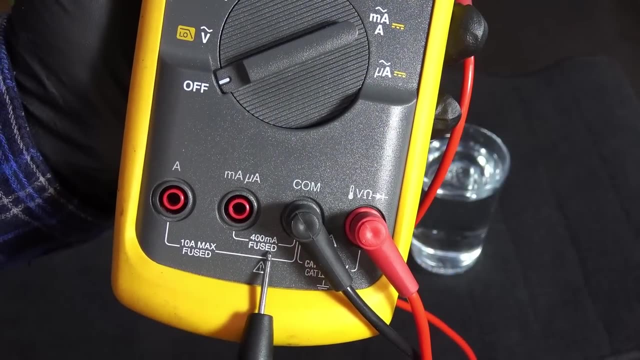 are lots of cheap but decent quality auto range multimeters available in the market. if you can try to find one with some useful additional features like reading temperatures, record peak values and safety features and so on, i wouldn't go much into it because those features aren't that. 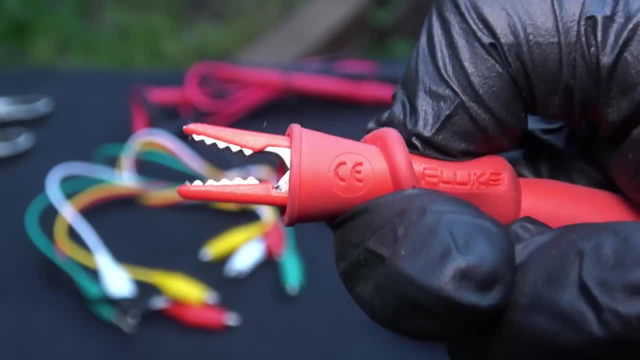 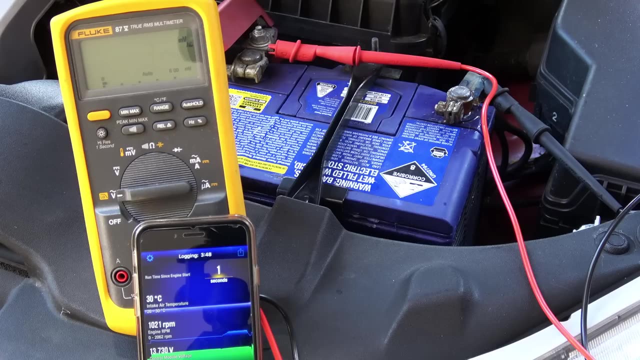 necessary when you first start out. last but not least, add some alligator clips and some jumper wires for your shopping cart, because this is gonna set your hands free when you need them. the next question you may have is where to buy a good multimeter and what is a good brand you can buy. 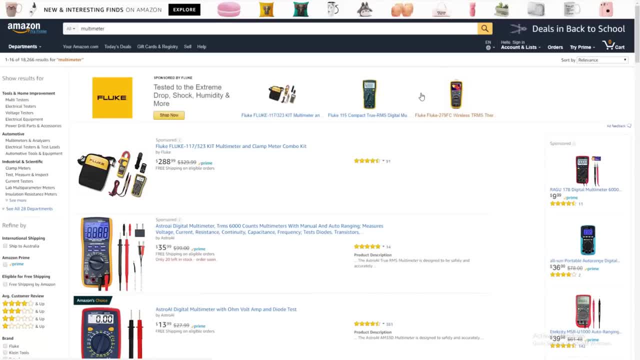 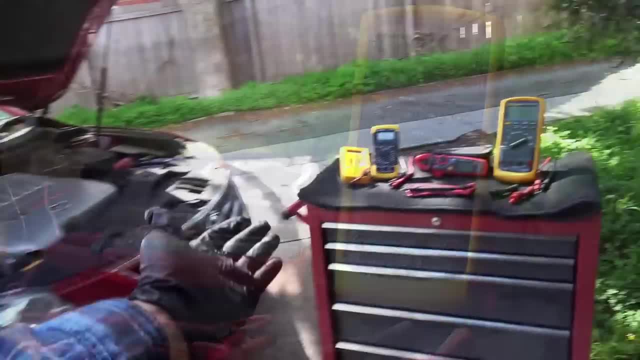 any good electronic shop or from online shops. speaking about the brand, good brands are often very expensive and those are mainly for professional users. so if you're a beginner, most multimeters in 50 to 100 range will serve your purpose. hopefully this video is helpful and if it,